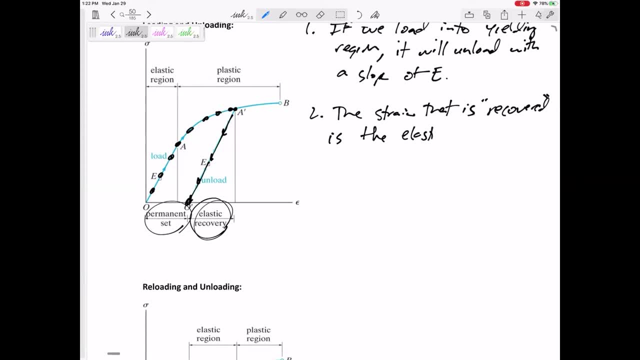 back from? is the elastic recovery, The strain left or the strain you know that is not recovered? is the permanent set or the permanent deformation? Okay, I like to call this our unloading triangle. The unloading triangle has a slope of E. 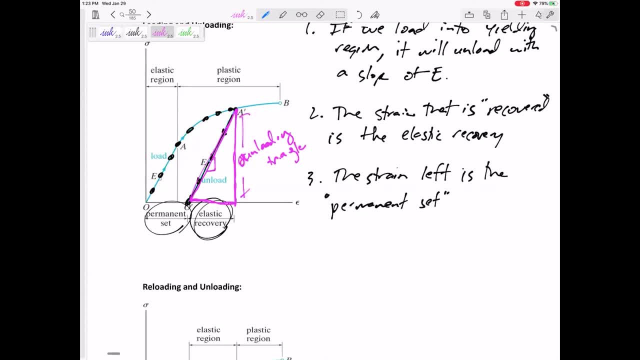 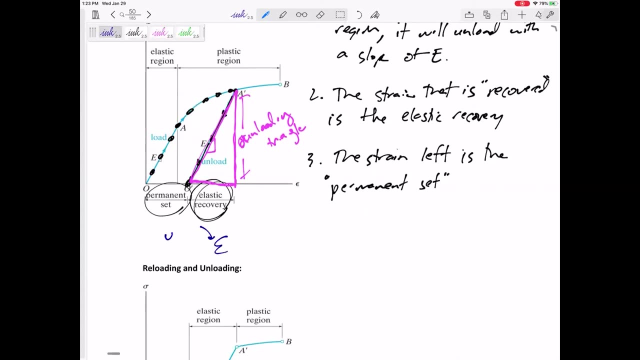 When this whole stress, this stress is let go. the base of that unloading triangle is the elastic recovery and the amount left over is the permanent set. So how about this? It's the strain when loaded. So this strain right here is equal to the permanent set plus the elastic recovery, right. 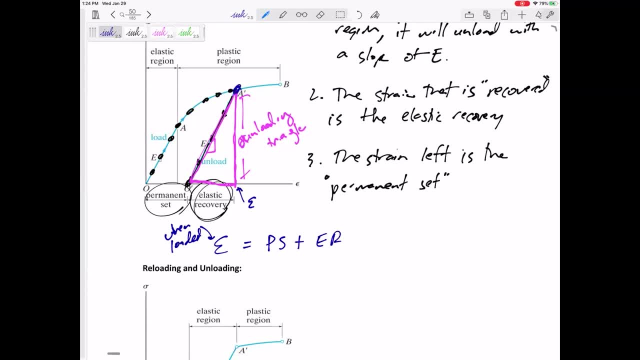 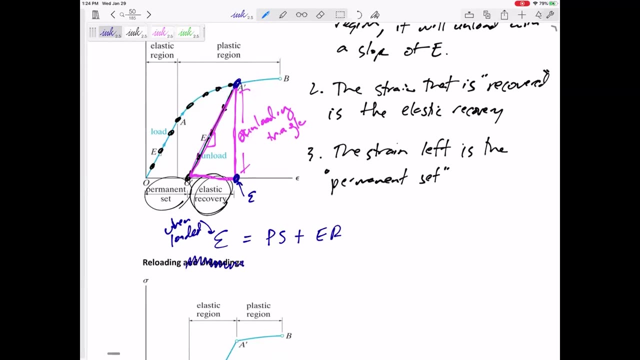 So if you know when it was loaded up here it had this strain of epsilon, You can calculate the elastic recovery and what's left over is the permanent set. Okay, if we were to do this up here, load it up here and unload it. 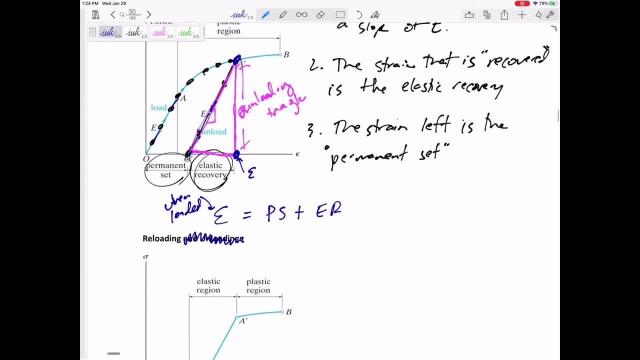 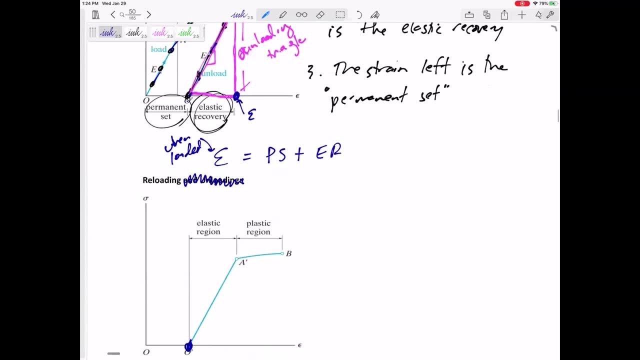 if we were to reload it again, it would be starting at that point right there, all right, And it would load up at a slope of E, and then it would go back and it would hit the old stress-strain curve. Okay, so it's almost like we kind of erase this portion. 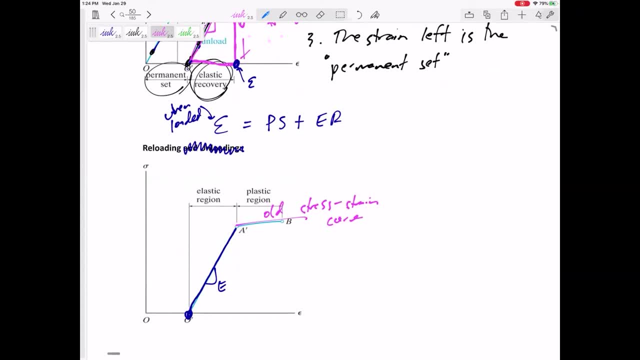 and we have a new stress-strain curve. So there are benefits to actually- and this is strain hardening right- There's benefits to actually loading something, stretching it and unloading it, because now you have a new stress-strain curve.